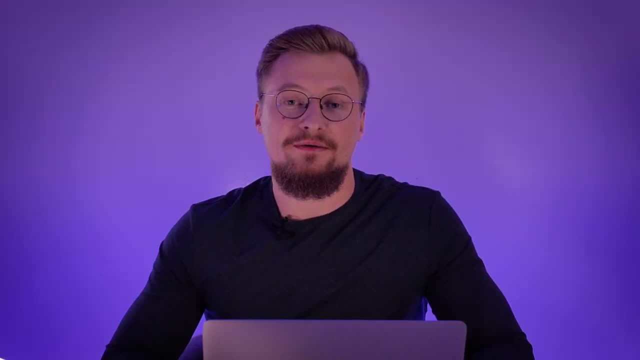 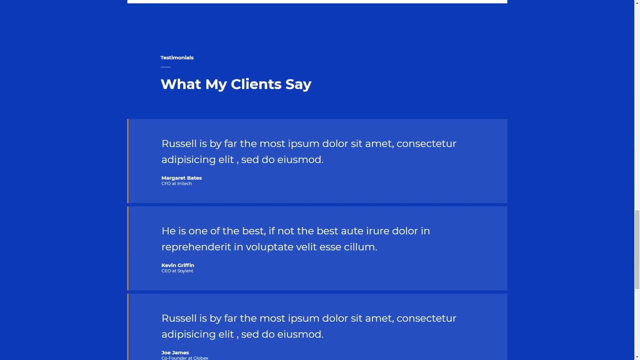 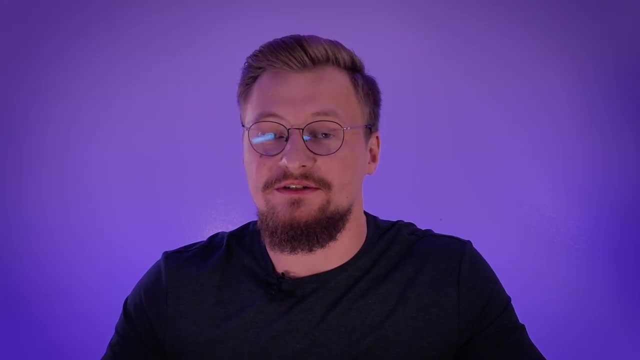 it's not crowded. Shared web hosting is a great choice for everyone who are building personal websites or blogs. It's also a really good option for small to medium sized company websites and considering other factors. it's cheap and you don't really need to know a lot of technical stuff. It's very easy to use. 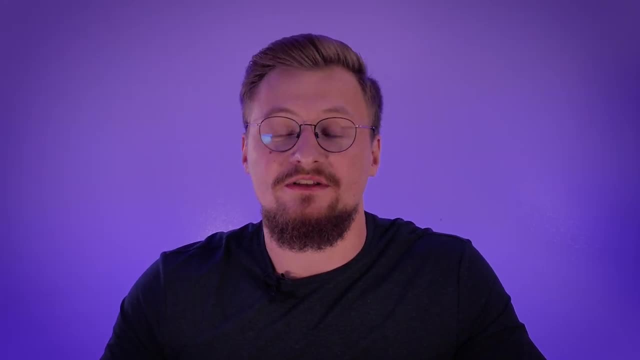 it's simple to set up and I would say it's the best option for beginners. And I have some good news: If you will use code HA10, you'll get 10% discount of your web hosting. So hurry up while you can, Since now you know the pros it's. 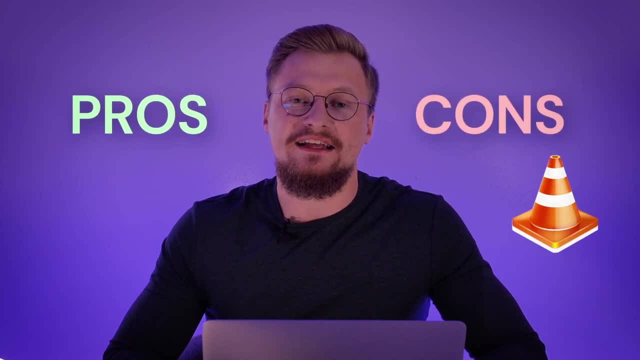 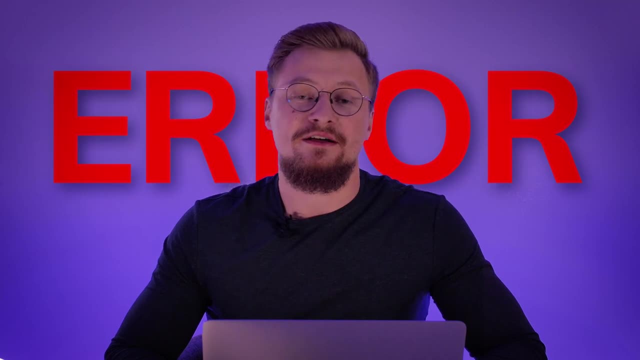 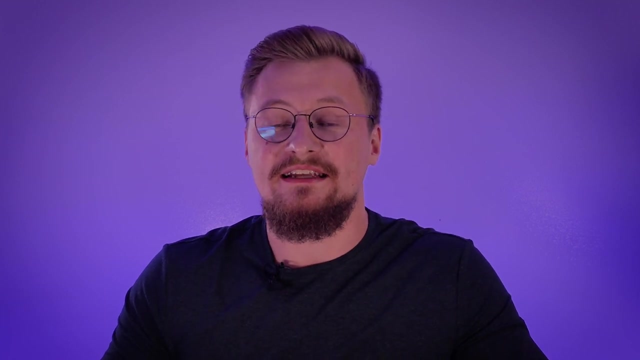 time to talk about the cons. Usually with shared web hosting you'll get less bandwidth and storage compared to VPS, and when there's high traffic you might experience some errors, But from my own experience I can tell you that this happens rarely. Besides that, you'll have limited access to the backend and it 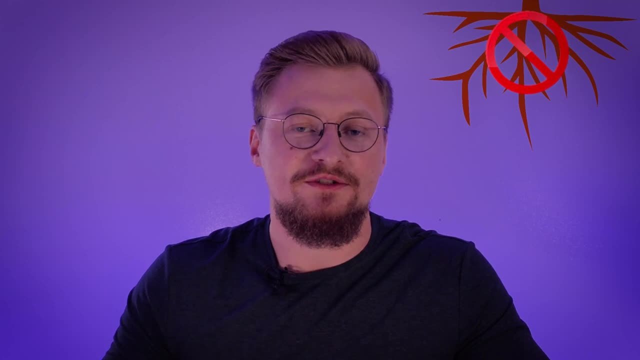 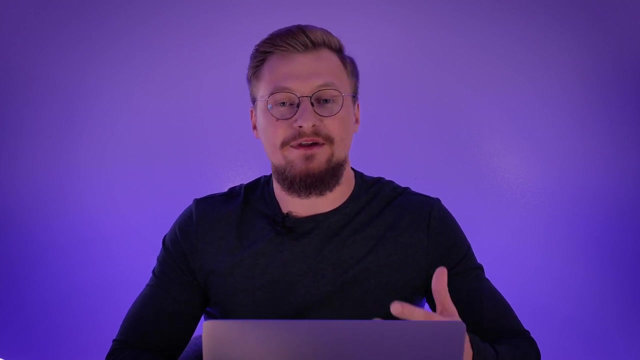 doesn't grant you a root access, But those things might be crucial to more experienced users. Alright, since now you know a little bit about shared web hosting, it's time to talk about VPS, Which stands for Virtual Private Server. You can even tell a lot from its name. 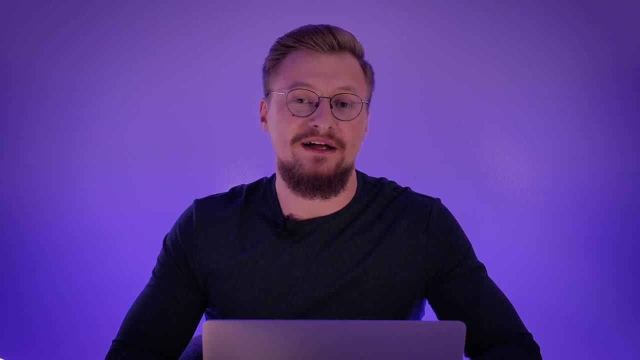 that it's the opposite of shared web hosting, because one is shared and the other is private. Instead of sharing resources with other websites, you will get dedicated resources. You will still be sharing one physical server, but each user gets specified set of resources. That's great, because other websites on the same server will not affect you. 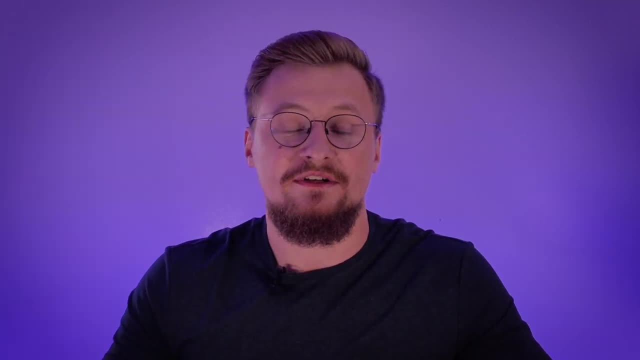 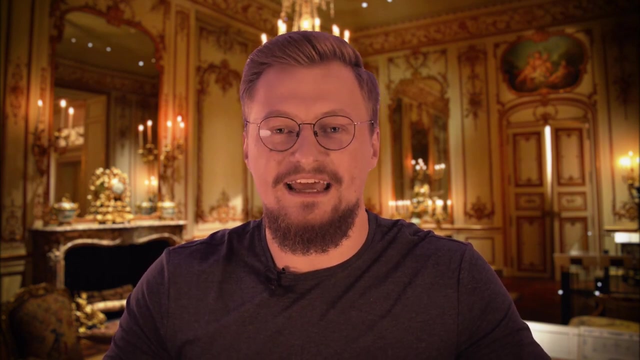 unlike with shared web hosting- Let's use the same example. So VPS is like owning a condo or a penthouse: Here you have anything you need and you don't need to share it with anyone else. VPS is a good option when you are running a business. 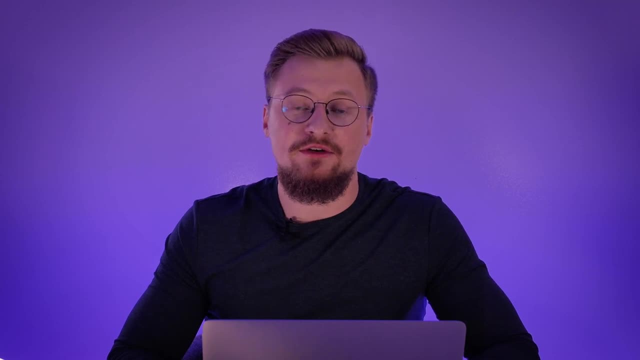 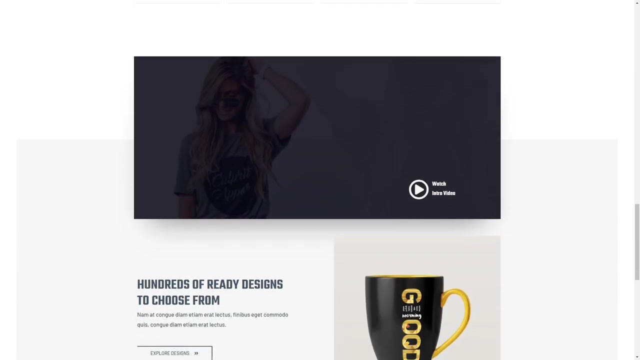 and you're planning to expand. It's also a good choice when you have more budget to invest to your website and if you are expecting high traffic to your website, you might also want to consider this type of hosting. All right, let's talk about the pros of VPS. Firstly, with